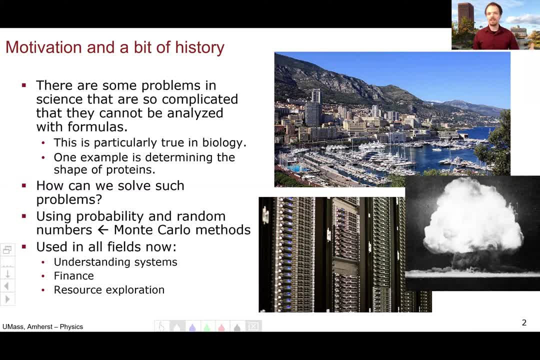 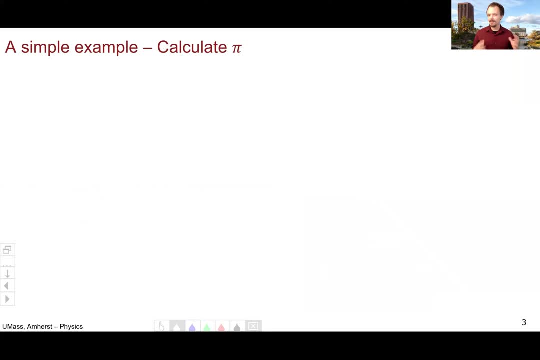 are commodity prices going to go up or down? resource exploration, like oil and other minerals- All of these different fields use Monte Carlo methods now to gain a deeper understanding of complex problems. As a first example of how Monte Carlo methods work, we're going to do something, maybe a little. 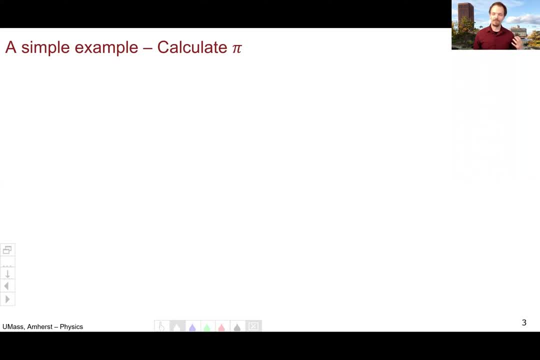 silly and calculate pi. So to see how we can do this using Monte Carlo, consider a square that's one meter on a side And inside we'll call this direction x, the horizontal and the vertical direction y, And inside the square, 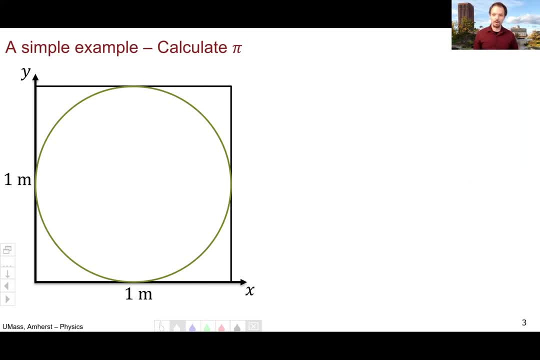 let's put a circle, And since the circle is one meter in diameter, it has a radius of half a meter. Now the area of the circle divided by the area of the square is pi, r squared over s squared. In our case, the radius is 0.5 and the side of the square is 1.. So the area of the circle divided, 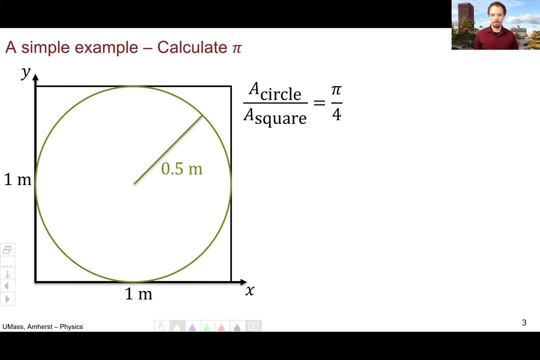 by the area of the square is going to be pi over 4.. So now let's use a Monte Carlo method to determine the value of pi. So how do we do this? First we throw a dart, or in a computer we choose a random x and y value. So in this first dart we got a very large x and a very large y. 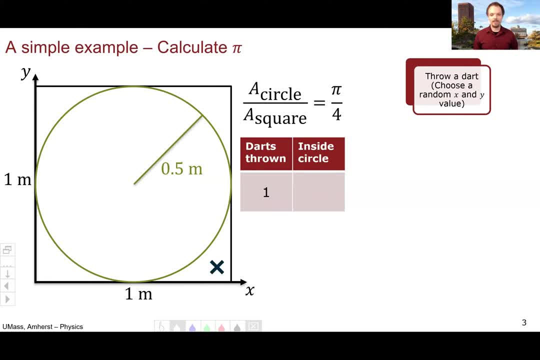 you can see it down in the lower right there. Then you check to see: is the dart inside the circle? I mean, if you're doing physical darts you can actually see. but if you're doing calculation, well, you do x squared plus y squared, Is that less than 0.5?? If so, it's inside the circle. If not, 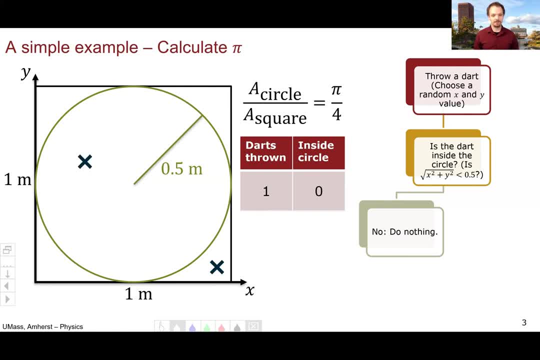 do nothing, Throw another dart. Repeat the process. This dart is inside the circle, So we add one dart for inside the circle. If you do a bunch of darts, the number of darts inside divided by the number outside will be the area of the circle divided by the area of the square. Think about: 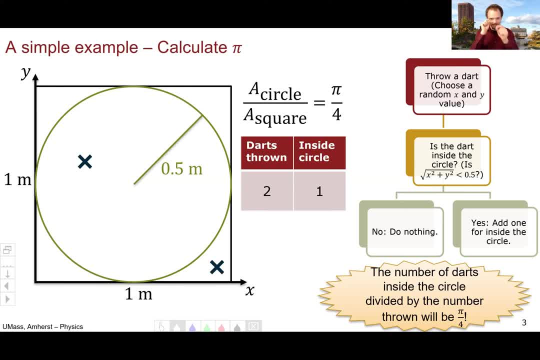 it in terms of probability, right, You're throwing darts at random. The number of darts that land in the circle, divided by the number of darts that land in the square, is going to be the ratio of their areas, which we've just seen as pi over 4.. If you do this for a bunch of darts, a bunch of 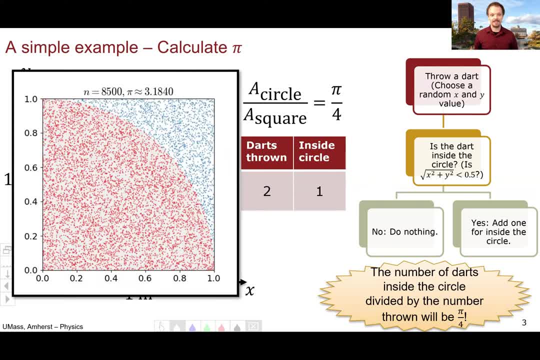 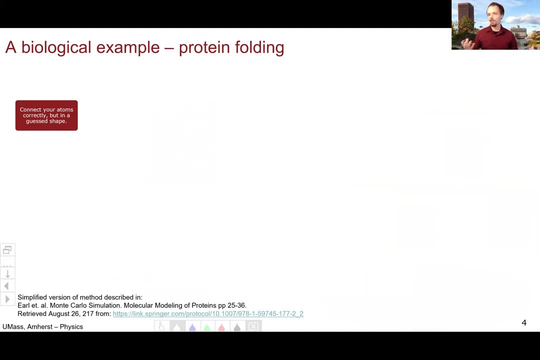 dots in a computer you can see that once you get to a couple of hundred thousand you start to get a relatively reasonable approximation for pi. So that example is a little silly. Let's do something a little more, probably interesting And a biological example: Folding proteins. This is, like I said, a famously difficult problem. 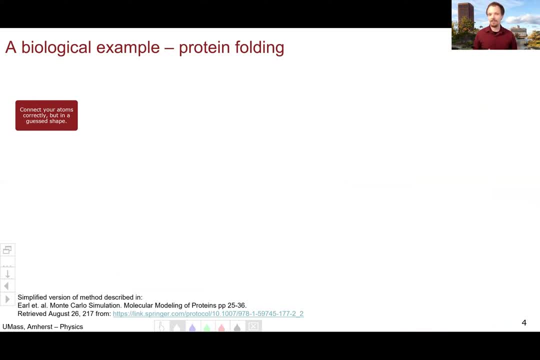 So here I'm going to take you through how you can use Monte Carlo methods to solve protein folding. The example I'm going to go through here is a simplified version of the method described in Earl et al. So how do you start? Well, you correctly connect your atoms in some random 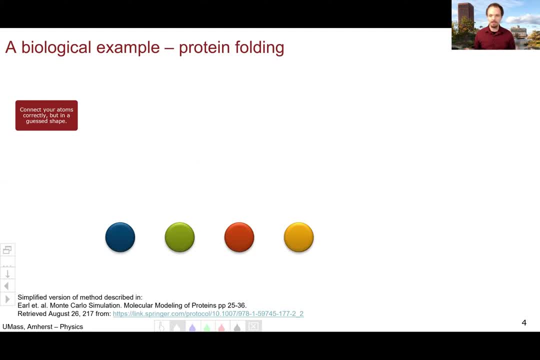 guess shape a straight line. I mean, if you can make a better guess, maybe you do, But if not, straight line is fine. The next step is choose a random atom and move it a small step in a random direction. So I'm going to move this green atom just up and to the right just a little bit. 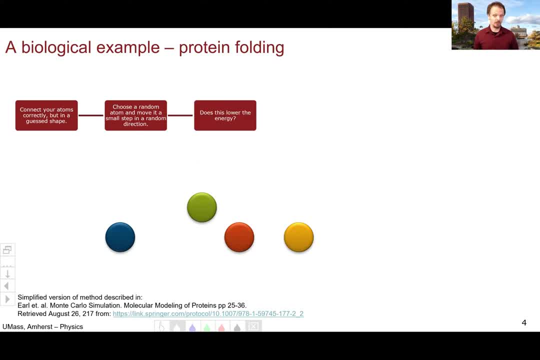 Now go and calculate the energy. Is this energy lower than the energy that you started with? If the answer is yes, leave the green atom where it is and start over. Choose a different atom. So now we're going to take the blue atom and get it to move. I'm going to move it just down the line. 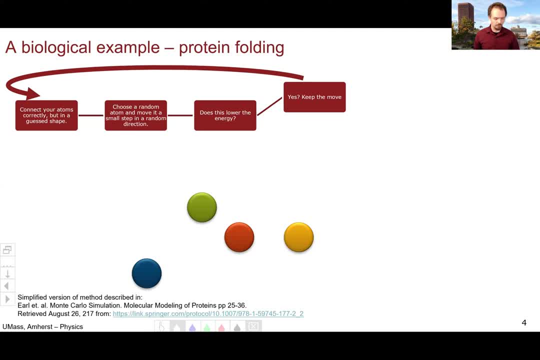 To the right a little bit. So we've now moved the atom, We go through, we calculate the energy. You'll actually see how to do this in the third unit of the lecture portion of this course. And let's say this time that no, it doesn't lower the energy. Well, you don't automatically move the. 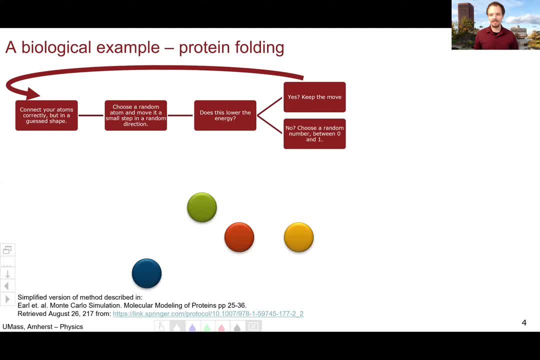 atom back. You choose a random number between zero and one. And why do you want to do this? Well, it has to do with energy Right. For all we know, our goal is to get to the lowest possible energy state in this situation, 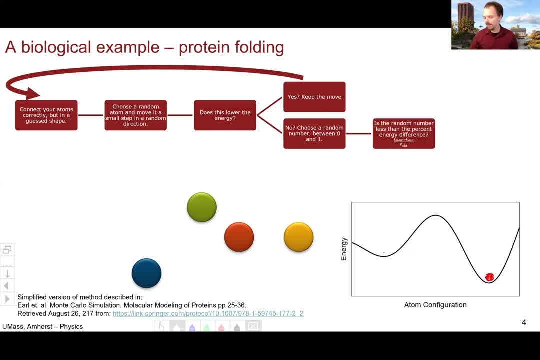 down here. But for all we know, moving the blue Adam got us here. So that's not the lowest possible energy state. So we choose a random number between zero and one, And then we compare that random number to the percent energy difference. So the new energy.